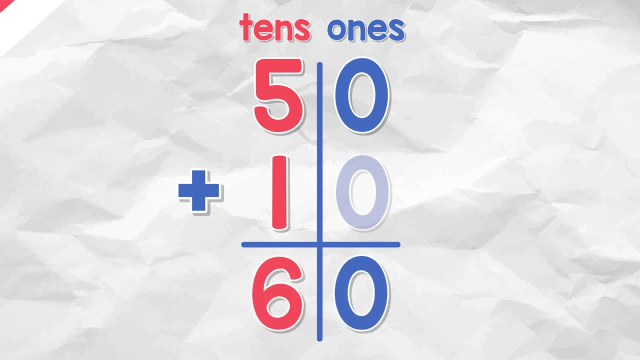 You get number 60. This is number 60 at a 1 to the 10s place. You get number 70. This is number 70 at a 1 to the 10s place. You get number 80. This is number 80 at a 1 to the 10s place. 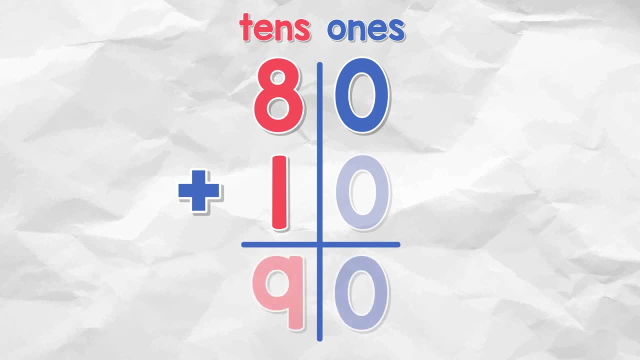 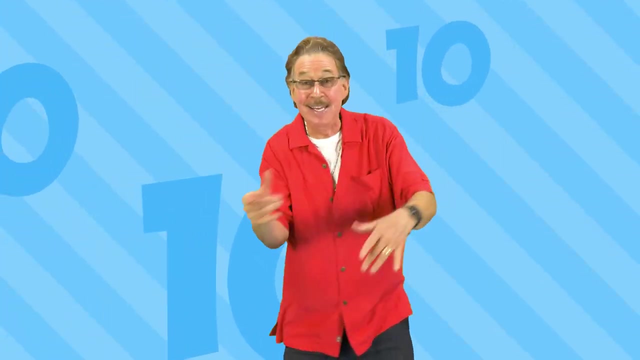 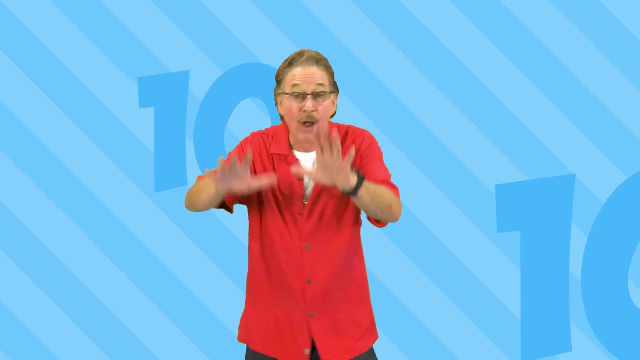 You get number 90. This is 85. Add a 1 to the tens place. You get number 95. Count by tens from any number. Count by tens. I'll show you how. Count by tens from any number. Count by tens. let's practice now. 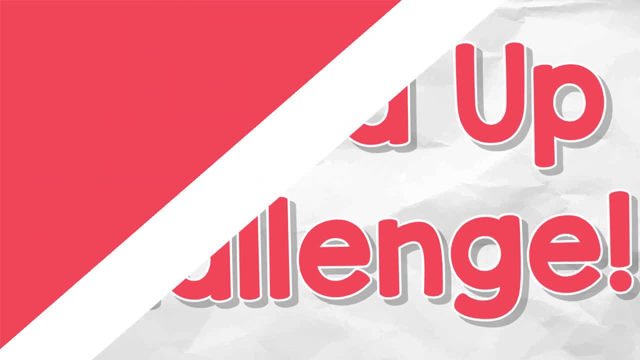 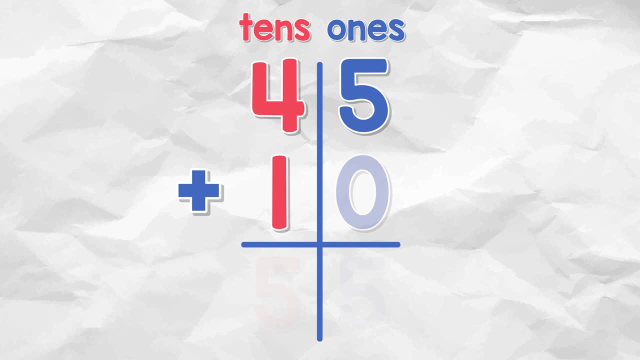 Get ready for a bigger challenge. This is 45. Add a 1 to the tens place, You get number 55. This is 67. Add a 1 to the tens place, You get number 77. This is 32. Add a 1 to the tens place. 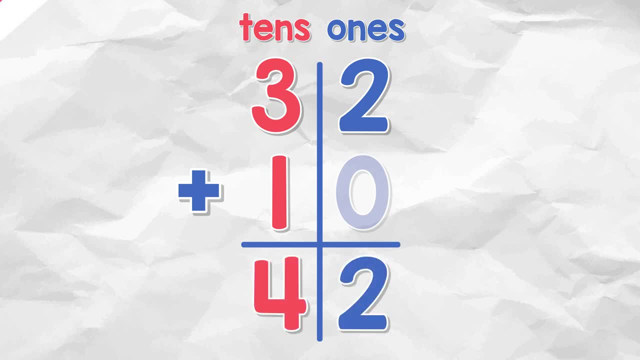 You get number 42. This is 17. Add a 1 to the tens place. You get number 27. This is 72. Add a 1 to the tens place. You get number 82. This is 51. Add a 1 to the tens place. 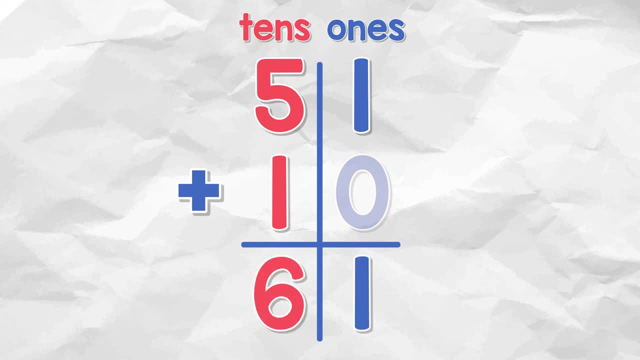 You get number 61. This is 84. Add a 1 to the tens place. Add a 1 to the tens place. You get number 94. This is 26. Add a 1 to the tens place. You get number 36. This is 89. 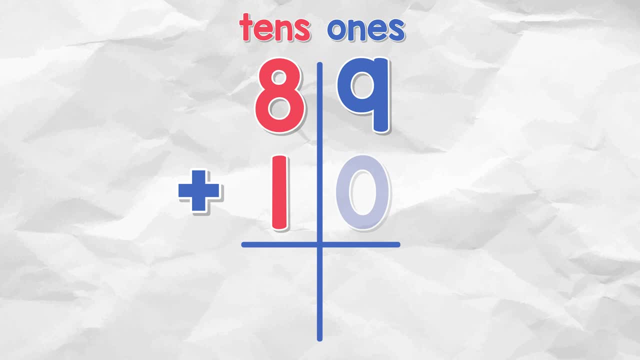 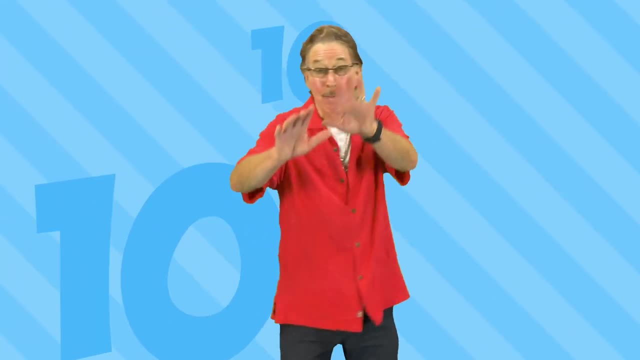 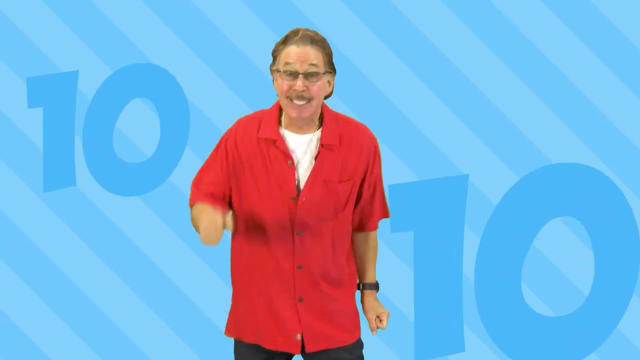 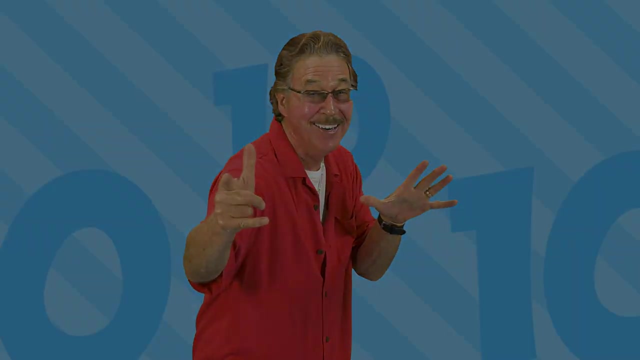 Add a 1 to the tens place, You get number 99. Count by tens from any number. Count by tens. I'll show you how. Count by tens from any number. Count by tens. you did it, wow.